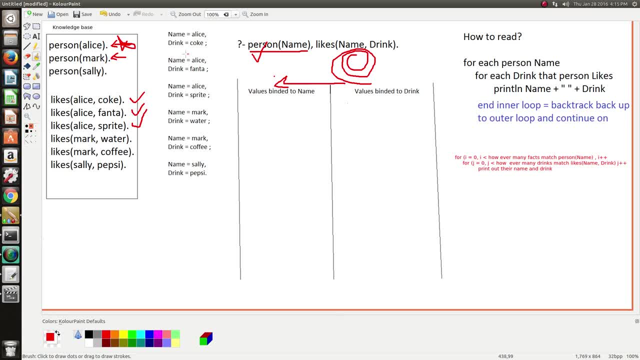 fact to evaluate. And then it's like for every drink, Mark likes iterate through his drinks: Done, done And kick back. And then prologue goes back here. We increment the counter again, um to simulate uh iteration and then it would go back to uh. continue on to Sally. 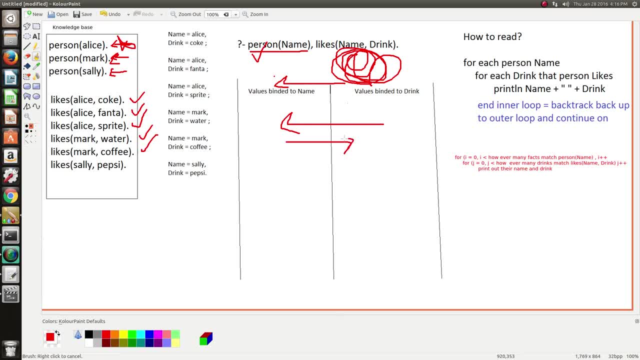 and then it would be like: okay, for every, every drink Sally has iterate, okay, that's the only drink Sally likes, so then we kick back, but then Prologue has no more of the outer loop to process, so the outer loop ends and therefore the whole thing ends and eventually 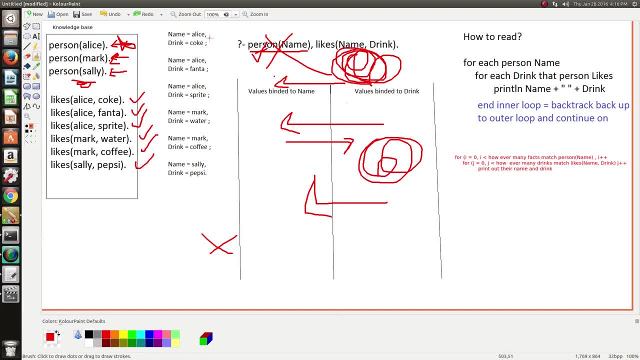 you end up with this and you can sort of see this pattern because, um, uh, for every, for every name print out: drink their drinks. and Alice has, she likes Coke, and then she likes Fanta, and then she likes Sprite, and then um Prologue backtracks up and it finds: 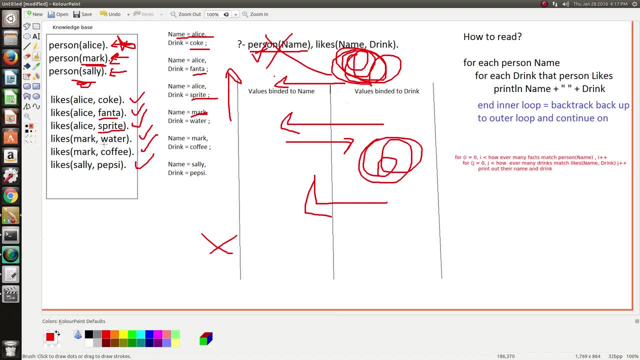 Mark. for every drink Mark likes, print out what he likes. Mark likes Coke, Mark likes Coke. Mark likes water, then Mark likes coffee. okay, backtrack back up. then we're back up to Sally. Sally likes um, Pepsi. no more drinks that Sally likes. so then we backtrack. 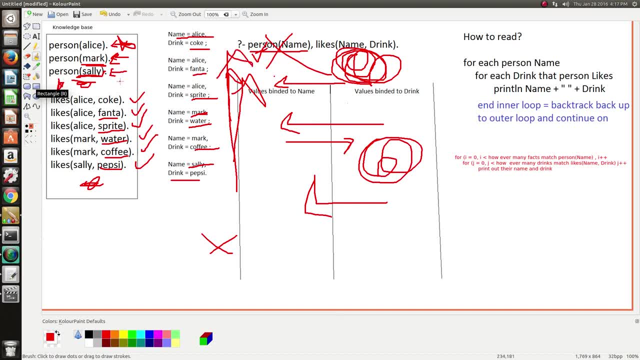 back up, but there's no more people, so we're done, And that's the simple list explanation I can give you. um, and I tend to think of it like like two nested loops in Java or something, and this is basically essentially what I was. 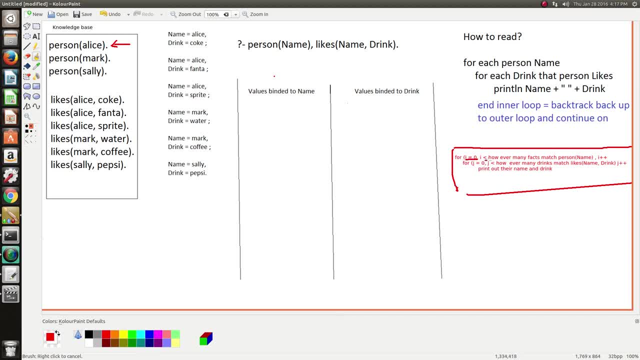 saying: for every person, um loop, the outer loop loops however many people there are in the knowledge base. and then for every person we loop through, we start an inner loop and however many drinks that that person has, that's how many times we loop through the. 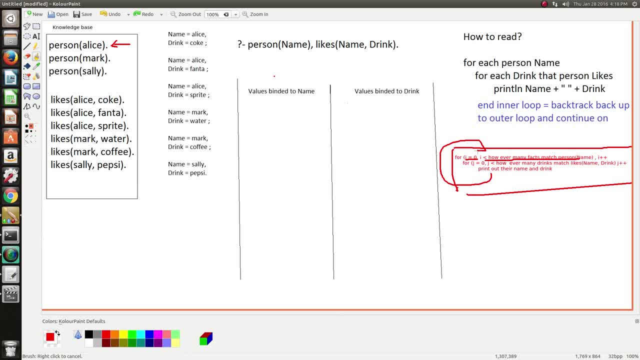 inner loop And then when the inner loop ends, we go back up. which increments i, which consequently will bring us down to the next fact in the knowledge base that unifies with the goal. And I've got this little table drawn up here and I guess I'd just like to demonstrate one. 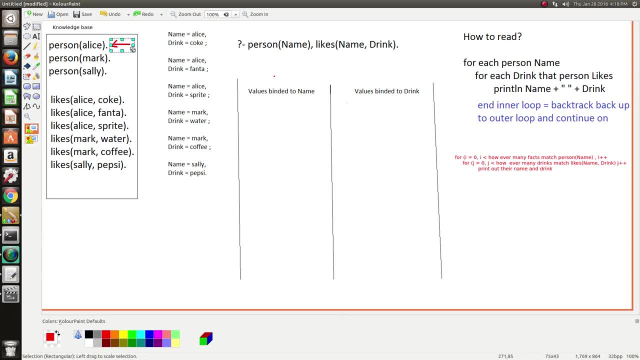 thing that is interesting and sort of explains the concept a bit more, Is that prologue will first to start off. it has this goal to achieve, so prologue will set up a marker here on the goal that it's actioning. so Alice is now binded to name. 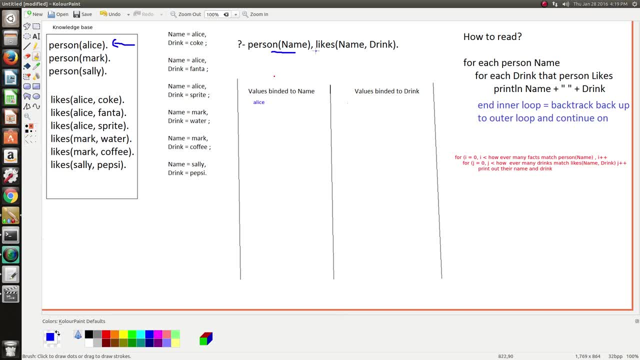 so it's working on this one now, and now it's gotta start the inner loop, so it's gotta work on this goal. So what prologue does is The values binded in goal will, And that's what I keep saying. 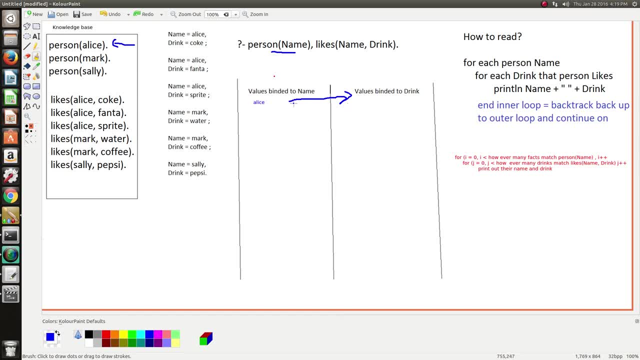 one of pass three to goal two. So think of this as like a pipe and Prolog passes through the variable bindings that it achieves in this goal. So in this goal we binded Alice to the name. So Prolog sends this through a pipe and it goes and visits the next goal. 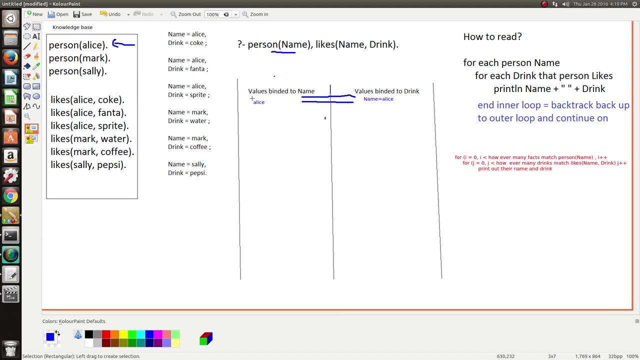 because the next goal needs the values obtained, the bindings obtained in the previous goal, to derive what drinks to look up for that certain person. So this means that this goal here now establishes it now knows what names to look up in the knowledge base. So then it starts. it sets off another marker at Alice, because that's. 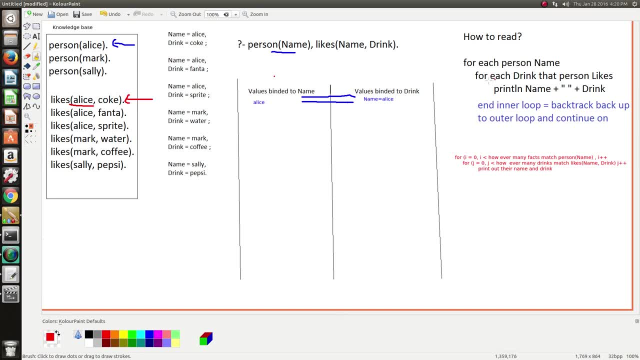 that's the name that we're looking for, and then it starts this inner loop here. so then it prints out: Alice likes Coke- okay, we're done there. and then it will iterate through the next one. Alice likes Fanta- done. and it will iterate through the next one- Alice. 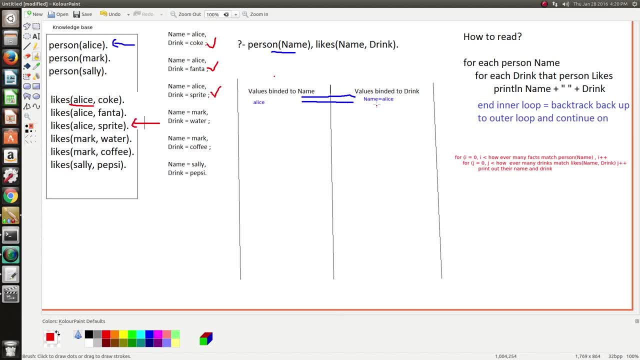 likes Sprite. we're done. and because we're done here, Prologue will be like: okay, I have exhausted all the facts in the knowledge base that unify with this goal based on the name Alice. so it kicks back and backtracks back to the first goal, so we can just remove. 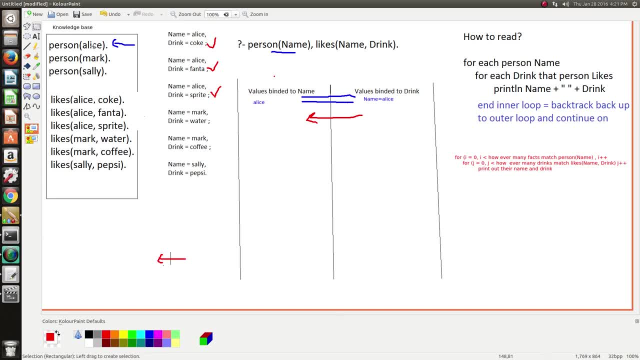 this pointer here, because we're not doing that anymore. so then Prologue's back into this goal. so then it goes down and scans the next item or the next fact. So in this process, in the backtracking process, any values that were previously binded. 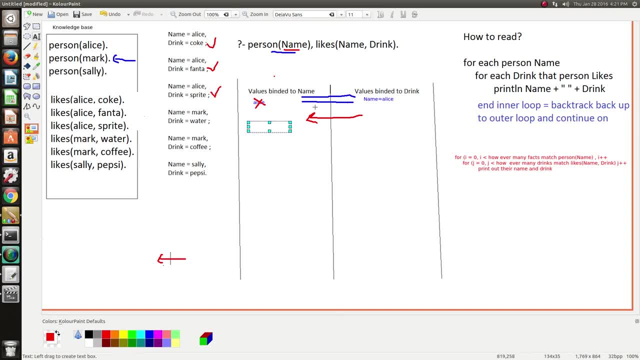 to name are erased so we can assign name a new value. so now Mark is assigned to name and, like before, we set up this pipe or tunnel leading to the second goal and we're done, okay, And we've binded, name equals Mark, so we can send this through the pipe to the goal. 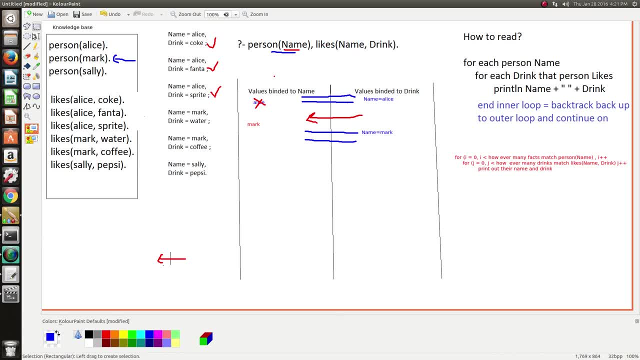 too, so that they know what name to look up. so this is when Prologue then establishes a new marker point. it scans through the knowledge base to find what drinks does Mark like, and it runs into here. so then it prints out: Mark likes water. 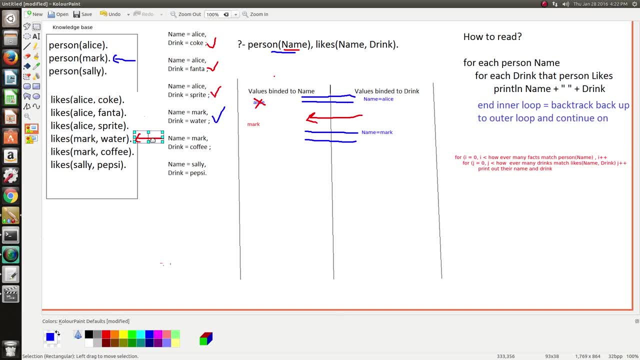 And it keeps searching for names that match Mark. then Mark likes coffee and we've run out of options for Mark, so we're done here, and then we don't have anything more, so we backtrack back to the first goal. that means Mark is unbinded to the variable name, so 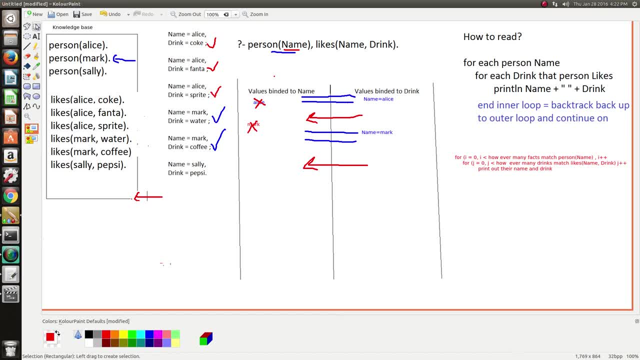 name doesn't have any value associated with it. So this means Prologue can bind another name to it. so it moves the marker down to the next fact that unifies with this, and then now Sally is binded to name. so in that case,